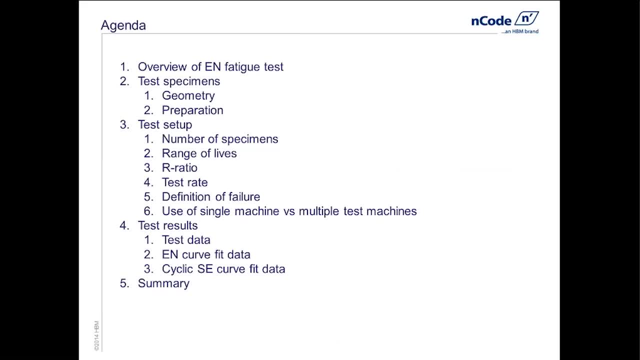 the key requirements. if you've asked to have a fatigue test done, the answers to questions that would be given to you, And so we'll talk about various test specimens, the overall test setup, look at some of the test results that will come out, and then we'll have a summary of what I consider to be the important factors driving this. 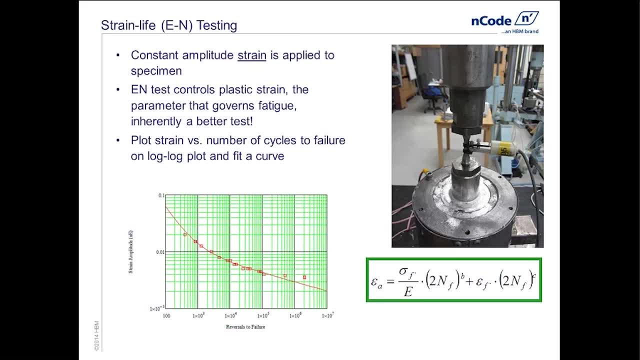 When we do fatigue, we have to be aware of the variety of different damage models we can use. We're going to focus on strain life or crack initiation and in order to do that style of analysis we need to have a strain life curve. The strain life curve is actually developed with a series of constant amplitude strain tests. We use strain life because it actually looks at total strain, elastic and plastic, tracking the plasticity. 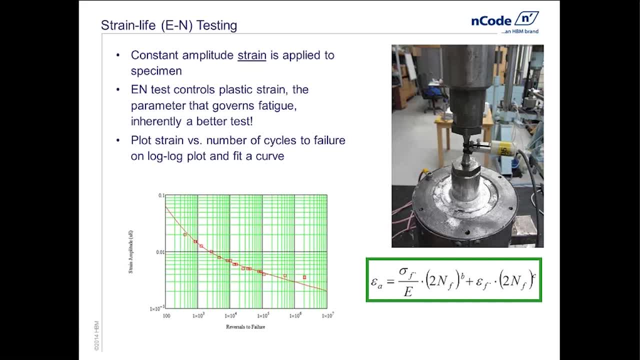 actually mimics the what governs fatigue and hence gives us an ability to do both low cycle and high cycle fatigue. It also gives us, because of plasticity, the ability to track residual stressors that occur due to loading. What we're going to end up with is the curve as we see down in the lower box. that is basically plotted on a log-log scale of 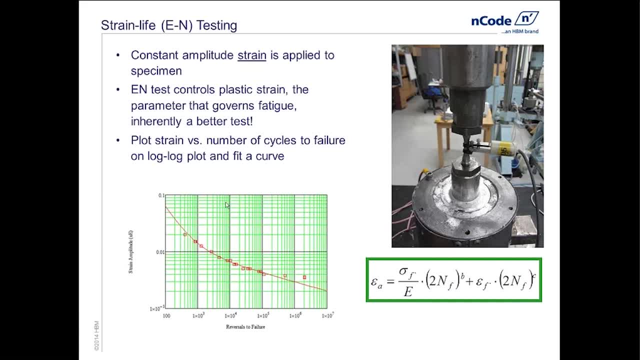 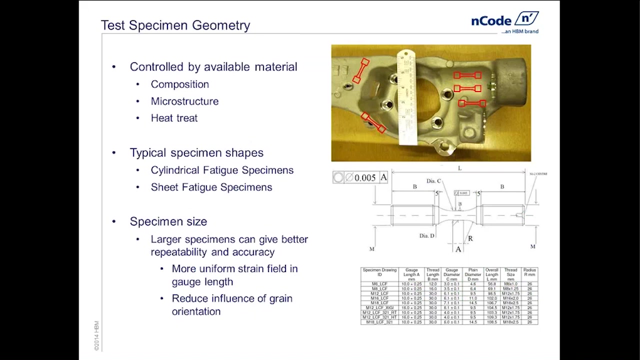 total strain amplitude and life, and that curve represented by this equation basically is going to be what we use for a fatigue calculation, looking at a combined low cycle, high cycle fatigue. those individual test data that you saw on the curve are basically tests we run on a specimen and the concept of this. 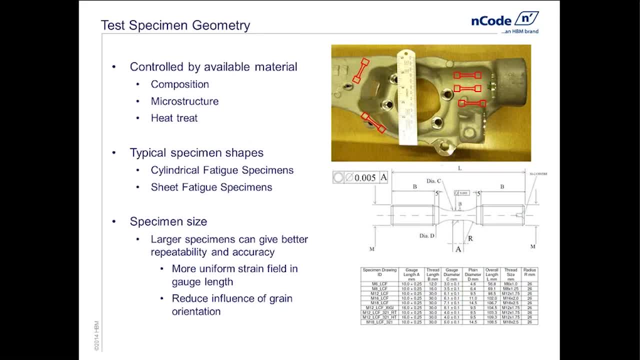 specimen. we want to generate specimens that represent as closely as possible our part. hence we want the specimens that actually have be made of the same composition, material, that have the same microstructure, the same heat, treat manufacturing processes as our part. now, with that that may actually control the 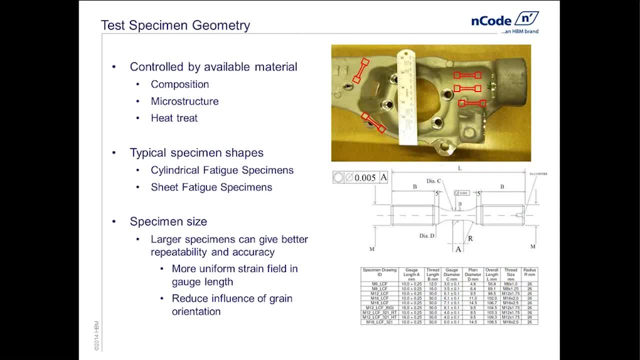 overall size of the specimen. as you see in the upper picture, we're trying to get a very small size specimen that can actually have sufficient. We have the ability to pull specimens out of our parts, but doing that is actually deriving the size of the specimen. 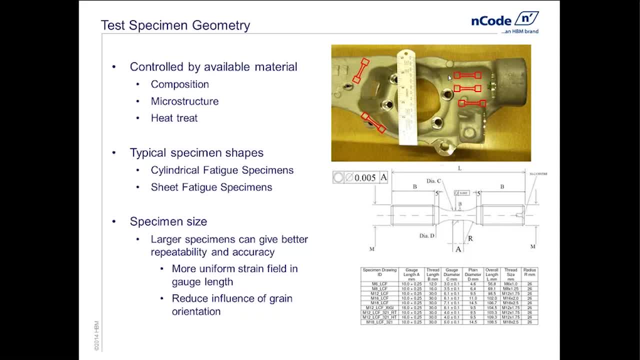 I've only got a certain amount of area that I can actually utilize. The overall shapes of the specimens are driven one by the part geometry, And so you'll see that there are typical specimens that are cylindrical, that would be used for things like rot or cast components. 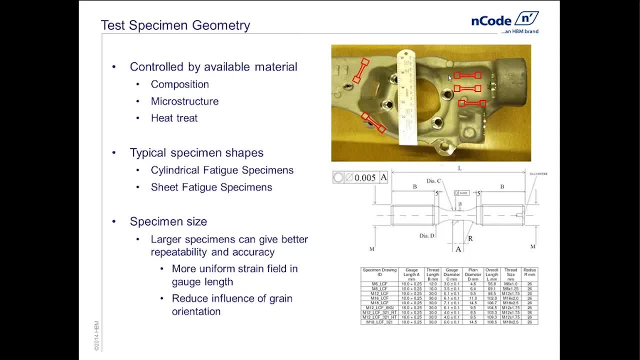 There's also flat sheet specimens that basically you'd use for things like roll stock. That's going to be pretty much driven by the material that you're working with And the specimens all tend to have standardized shapes. If you go to a particular lab, they'll have a set of specimen- shapes for both cylindrical and sheet specimens- that they would use. 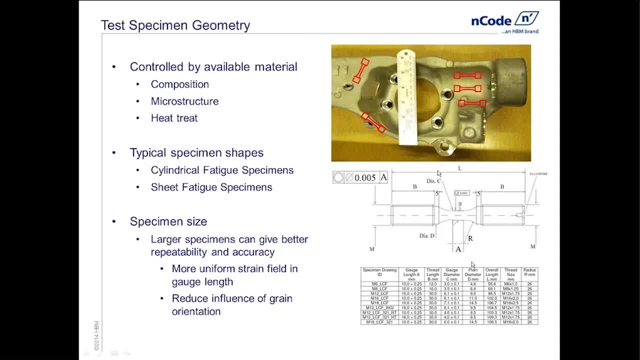 And what you see underneath the picture of the component is a schematic of a cylindrical specimen, And below that is actually a table of the cylindrical specimen sizes that we actually use in our lab in the UK. A couple things to note here. The end of the specimens are where the grips are gonna go on. 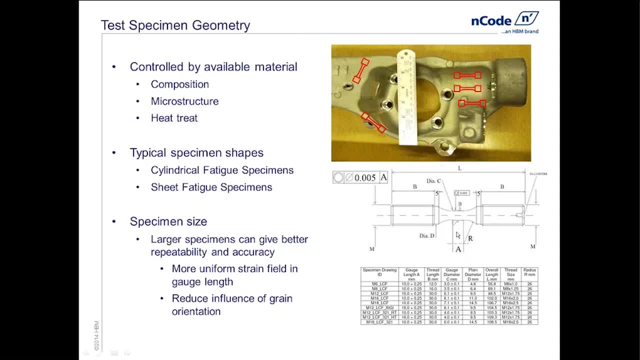 The key area is actually the center of the specimen. This designation A is showing you the gauge length. we're going to be measuring the strain at now. in terms of specimen shapes, they're pretty much standardized, but the sizes can vary and again, the size may be. 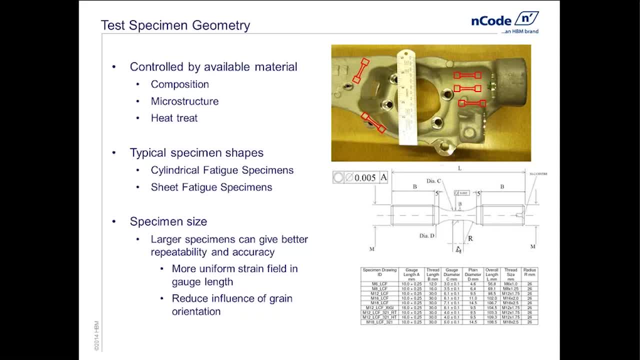 completely driven by the material that you're going to actually pull the specimens from. however, if you have a choice, a larger specimen size is desirable one. as we go to larger specimens, the gauge area, gauge length- is actually further removed from some of the geometry, those transition areas. 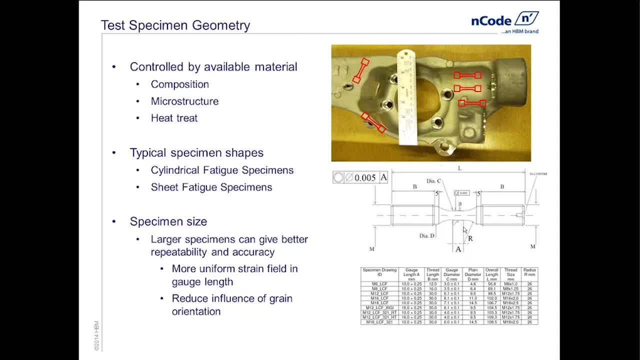 hence we can get a more uniform strain field. and secondly, even though the specimens may all look identical at the microstructure level, they are not, and as we have larger specimens, we can start to reduce the influence that the grain orientation has at the microstructure level and reduce some of the scatter. 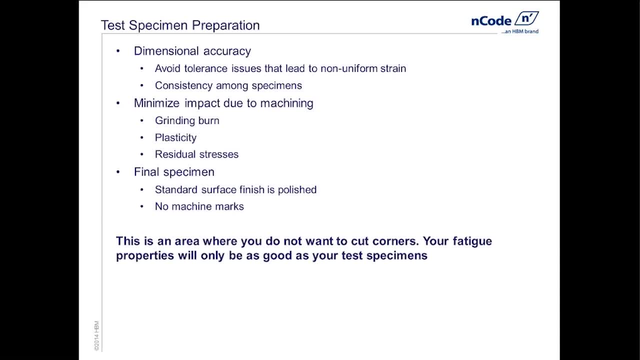 with the, the specimens. we now have to basically create these specimens from the material that we're going to be analyzing. and here is actually one of the key aspects: to get good fatigue results, the specimens one have to be dimensionally accurate. we're going to want to generate a uniform strain field in that gauge. 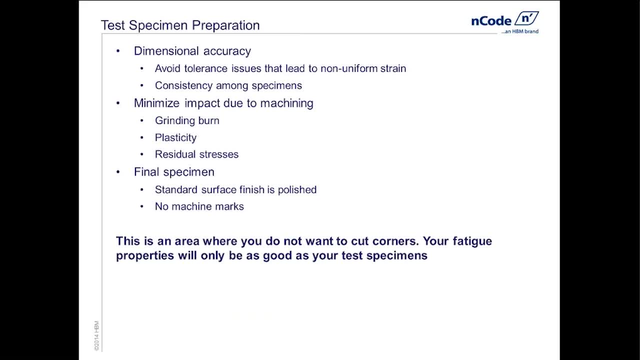 length and we're going to put it in the test we're using. we're putting under tension. we want these specimens to be able to generate uniform strain fields as well, the measure when we're measuring the spontaneous range or average years in a given case. so what we're looking at is concichtlich the 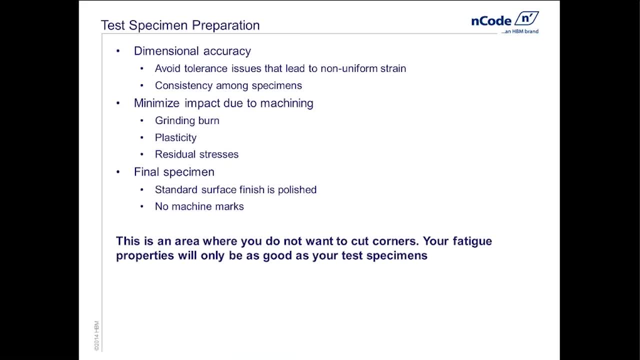 so we want to get those specimens manufactured. but how we manufacture them is also crucial. we want to create those specimens so we don't introduce any sort of plasticity residual stresses in the specimen from the manufacturing process. so we're looking to go in and be very 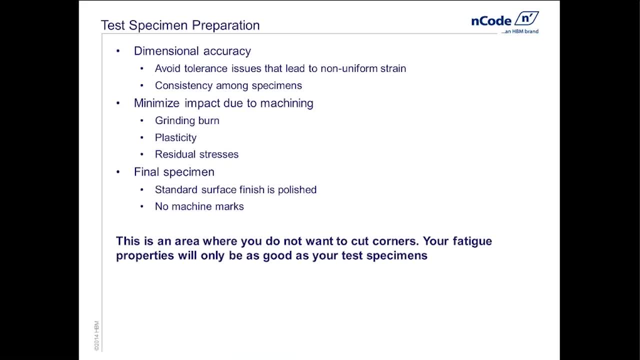 careful with the machining of that as we get close to the actual specimen shapes. we want our machining to be fairly light and use basically small cuts in the manufacturing process, sharp tools to try to go in and to end up with a specimen that has uh, minimized work, hardening. 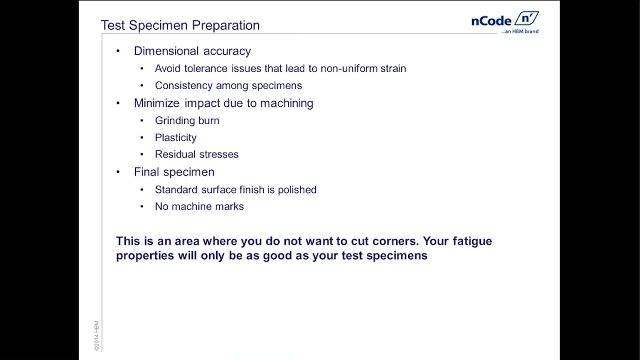 minimized residual stresses. also the final specimen: we want typically for the baseline curve to be polished. what we mean by that? we want the the surface to be removed of any machine marks, scratches. that would basically be introductions for the cracks. this is one place you do not want to try. 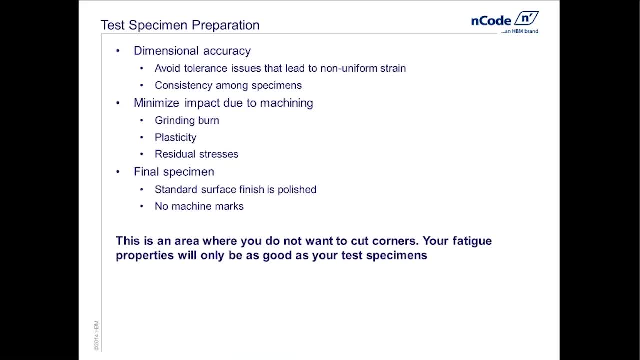 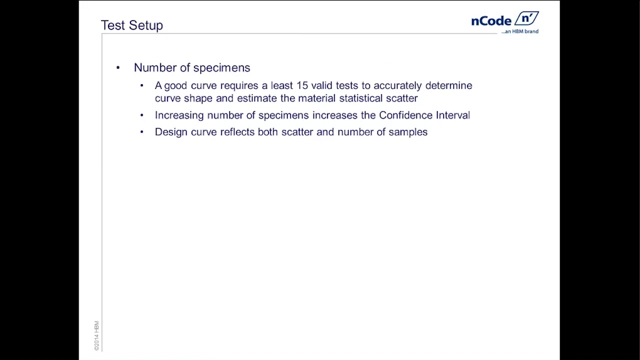 to cut corners. the specimen manufacturer is probably maybe around 100 a piece, but the quality of these specimens are going to completely drive the quality of the fatigue of the material and the quality of the fabric, and i think that's what we want: to make sure that we. 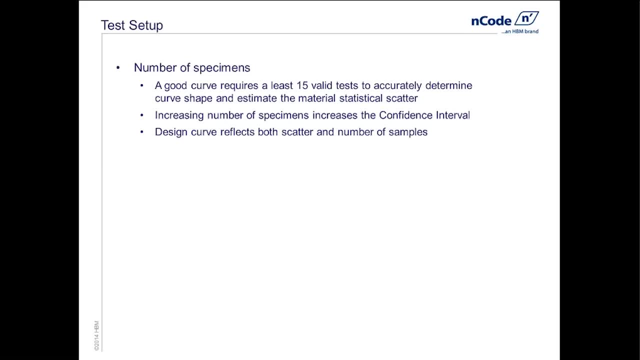 do is we have the materials that we need at the end of the year that are going to be used for machining, and the materials that we need to do it. we're not going to be making them right now. this is going to be a very simple calculation of the material that we're going to use at the end of 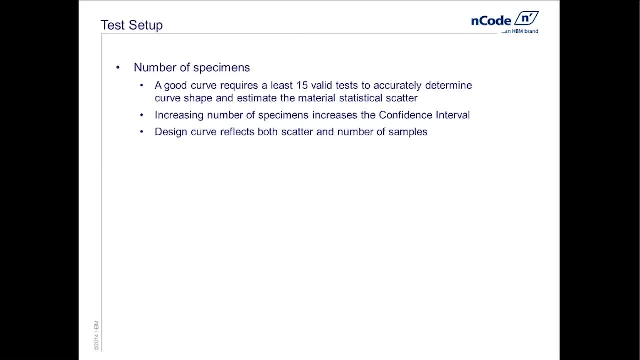 the year. this is going to be the final entrance for the. Are you going to use the basic material? Yes, we increase the confidence level we have in the data that we are looking at And we're going to generate a baseline curve that describes the average behavior of the material. 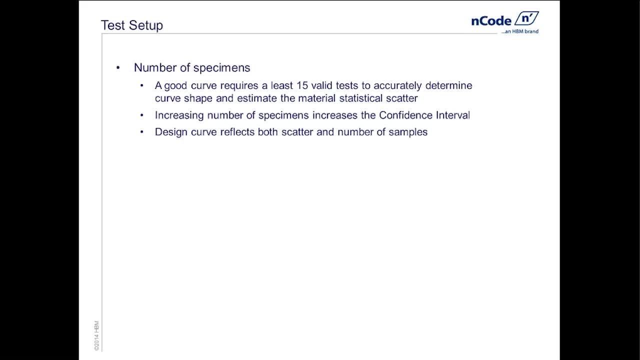 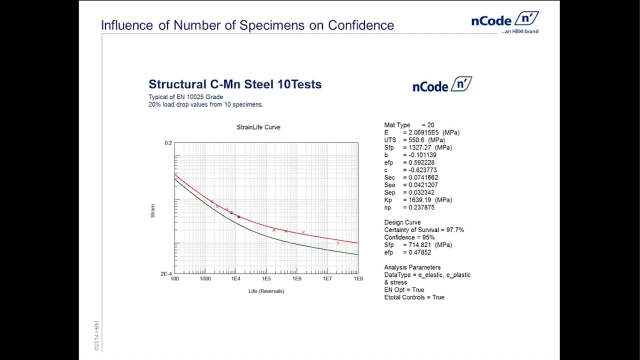 but in most cases you also want to derive a design curve that you can use that will talk about the entire population, a curve that we can design to And what I mean by that. here I have an example of a strain-life curve and if you look at the plot, the data points- both the blue diamonds as well as the green Xs- are actual test data. 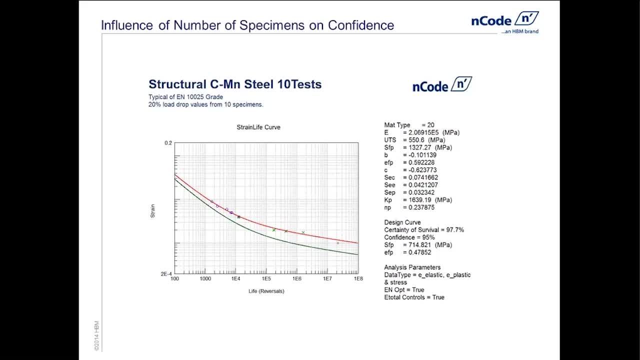 These are actually specimen tests. The red curve is actually the regression of our strain-life curve through that data And the red curve is actually the regression of our strain-life curve through that data, And you'll see there that we actually have scatter. Obviously, there is variation from specimen to specimen, even if they were at the same strain level. 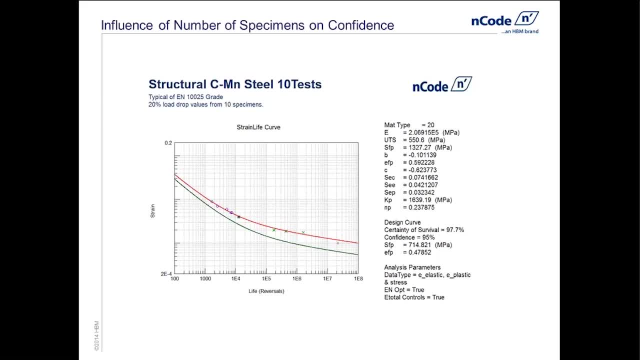 And that variation, that scatter allows us to go in and to quantify a certainty of survival for that curve, And so we have the ability to go in and, looking at the scatter, to shift the curve down, or actually we're always looking at high strain survivals. 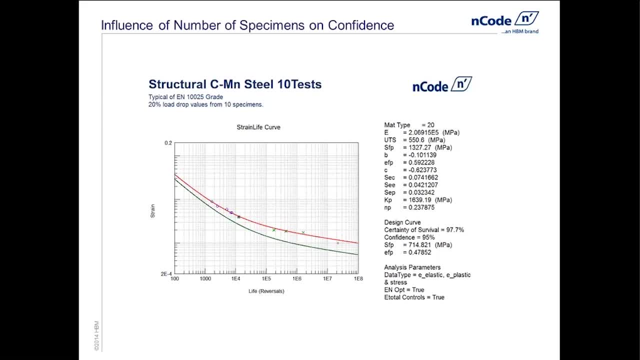 We're always shifting the curve down based on that scatter level. But there's a second issue with this as well. The curve that we're going to look to create is a screen curve. We call that the design curve, And that is not only a factor of the amount of scatter in our test data, but it's also how many tests that we had. 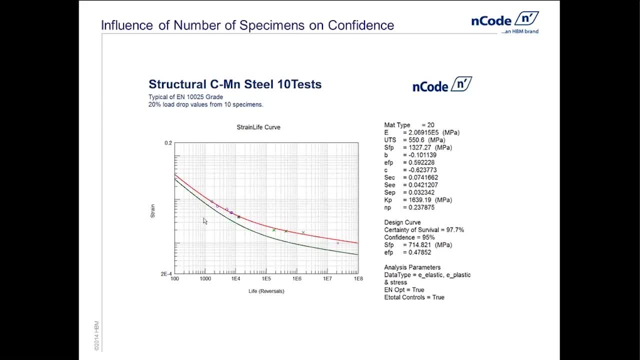 The more tests, the more confidence we have in our data and the stronger that curve is, the stronger that curve can be. In this particular plot, we're looking at a certainty of survival of 97%, which basically is two standard deviations shift down on the curve. 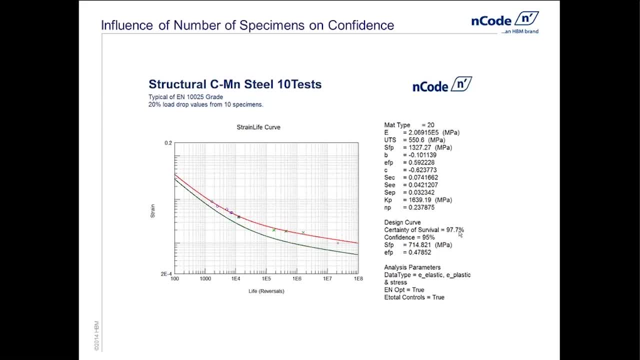 And we're looking at a confidence level of 95%. If I go in and increase the number of tests to calculate this curve, I can go in and improve our design curve. Since we have more confidence, we can actually use a less conservative curve. 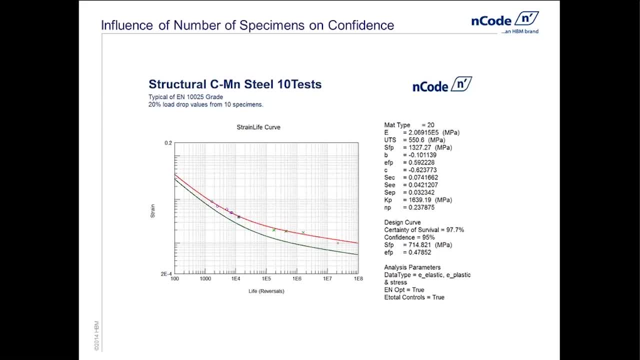 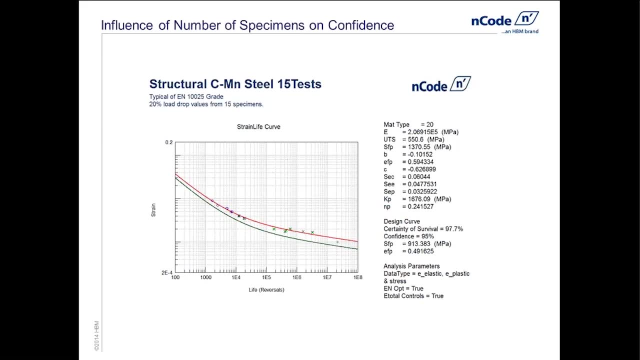 And so here we see a curve that's at 95% confidence using 10 specimens. If I go to 15 specimens, you'll see that the green curve has moved up. The design curve actually now is closer to the average properties because I have more specimens. 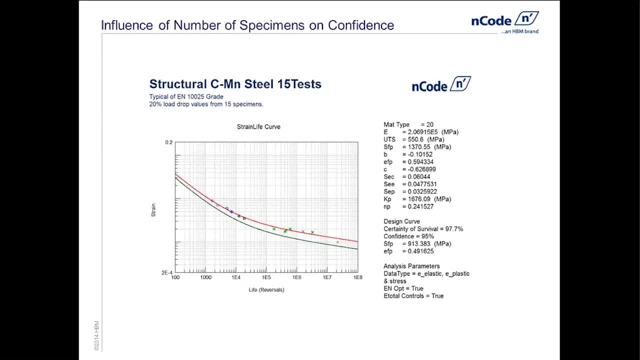 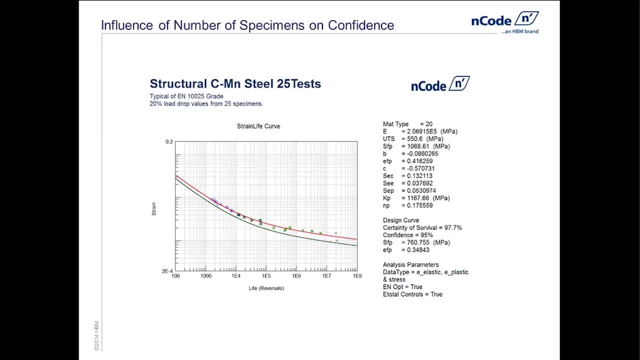 I have more confidence in the data And we have a final plot here that's looking at 25 specimens. Key aspect here: if I'm using this design curve, which typically we will be for our fatigue calculation- going in and trying to get away with a fewer number of specimens to reduce the cost of the test. 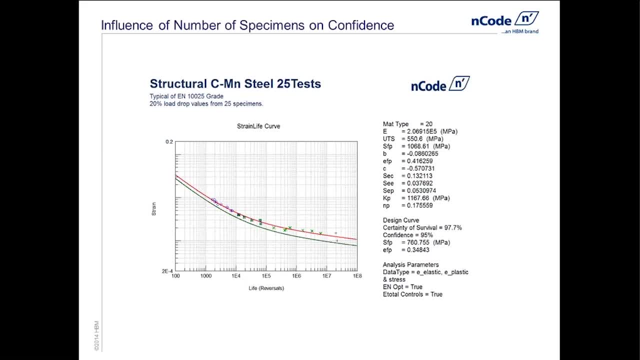 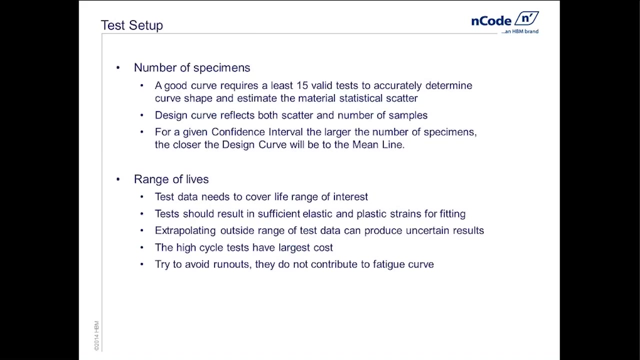 also gives us a design curve that is weaker. Hence we'll be adding more conservatism to the design, And the cost of that may be far greater than the additional test specimens. Besides the number of specimens, we also have to specify the range of lives that those specimens should cover. 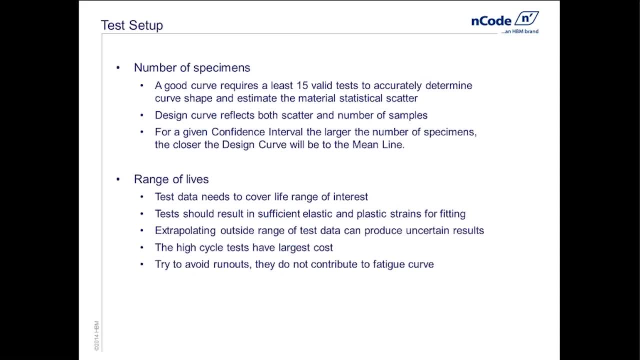 And what we need to do is make sure that we have tests that cover the entire range of life of interest. for our part, We also, when we develop these strain life curves, we're actually doing separate fits in the low cycle versus the high cycle. 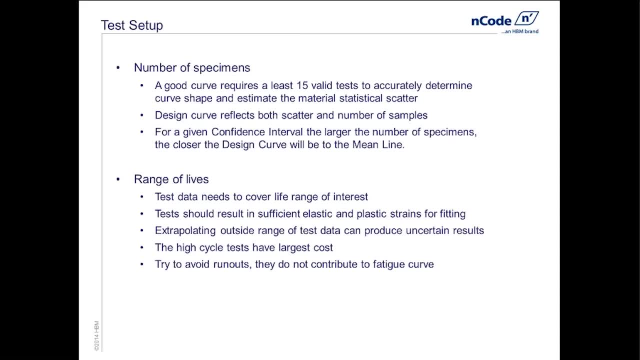 And we want to ensure that we have enough data points in both regimes, elastic and plastic, Thing we never want to do with these curves. we're fitting this curve through test data And extrapolation is very unpredictable. The curve has been defined by the test data. 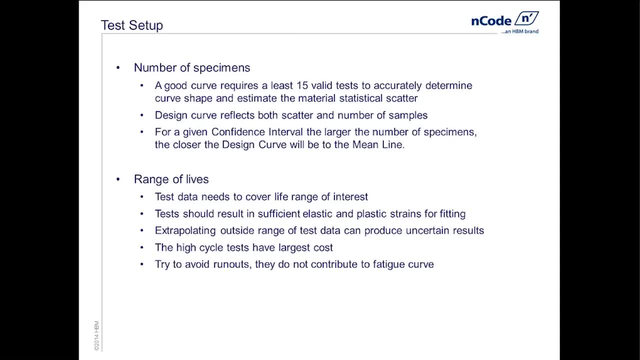 Areas outside the test region basically have no control. So we want to ensure that we're never extrapolating from that curve. We'll see that in just a second. The last couple things to mention: the test data from the high life, high cycle tests cost the most. 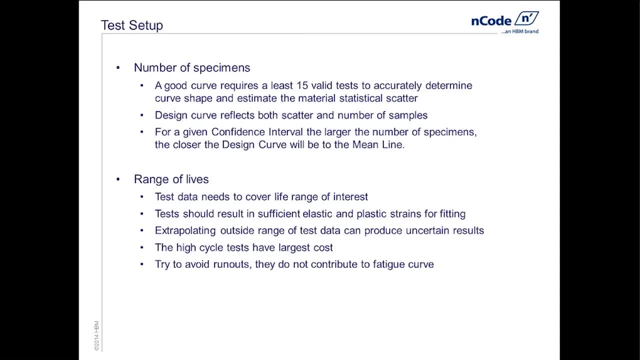 Those are the ones that run the longest. They're going to have the greatest cost, And so one way of controlling cost on a material test is to identify the high cycle regime that we're interested in, But not go much beyond that if we don't have to. 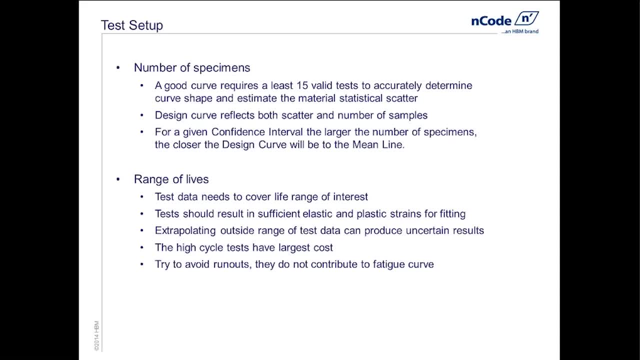 And in keeping in note with that, we want to try to avoid run outs. A run out is a test where we shut down the machine without failure And we've done that after we've hit a predetermined boundary life. you know, maybe 10 million cycles, 20 million cycles, something like that. 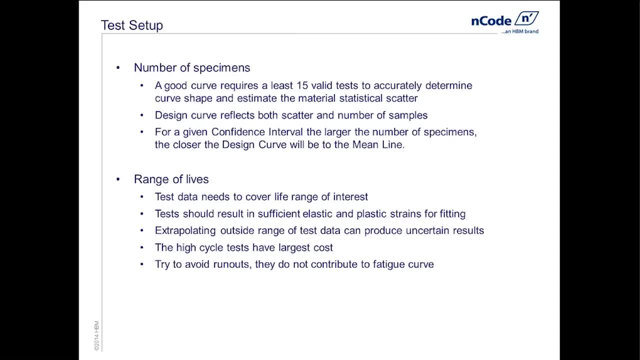 Where we basically say: at that point we're no longer interested in the data. One issue with that is that That's a very long test to that data point is not used in the determination of the fatigue curve, So it's a wasted data point. 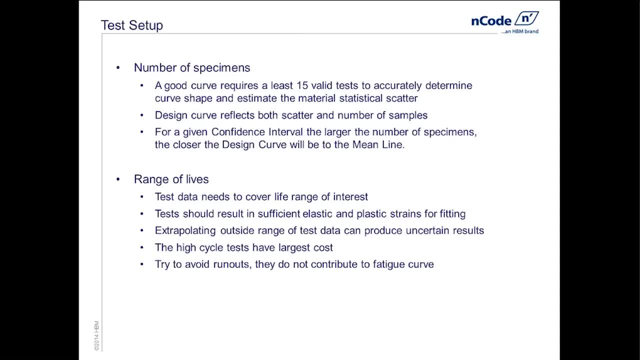 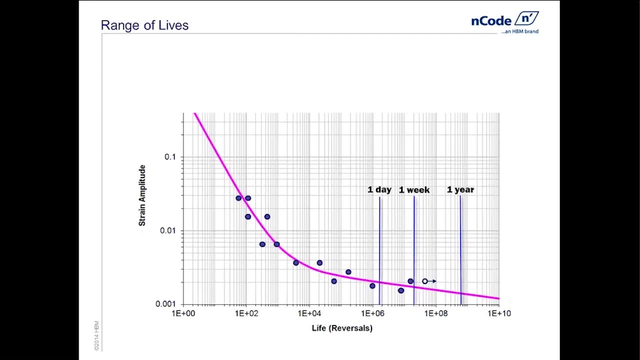 So minimizing run outs when we set up the test will give us the most efficient generation of a curve. Here we're looking at just kind of an arbitrary strain life curve And we're fitting through data, The blue dots. here are all data points. 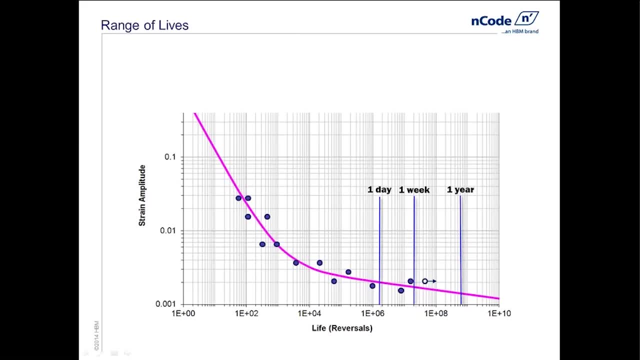 This one point out here With the circle and the arrow, is a designation of a run out. This is a test that we stopped here at looks like about 20 million cycles, So that was actually that test was terminated, And that data point isn't used in the determination of the strain life curve at all. 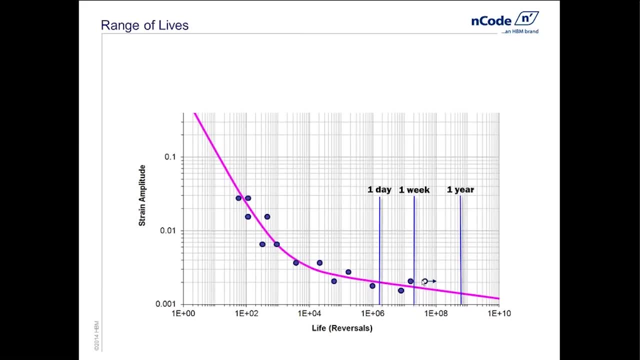 Now, one thing we want to identify is the valid range of data. What we've got here is a range of lies. I feel comfortable with this strain life curve As I go lower in life or higher in life. that curve is not being defined by the data. 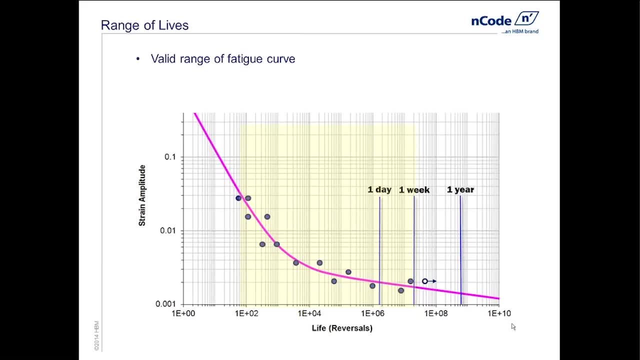 It may not be representing the actual behavior of the material at all, So we do not want to go outside that range. The other thing to note here Is we are going in and running a test at specific speeds, And we'll see that in just the next slide. 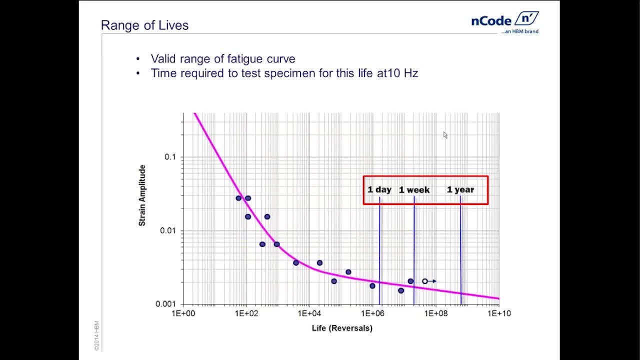 But at that test speed it takes me a certain amount of time to hit life, Hit the life target life that we're running. And one can see here, just as we start looking at the high cycle data, That if I'm sitting out here, just under a million. 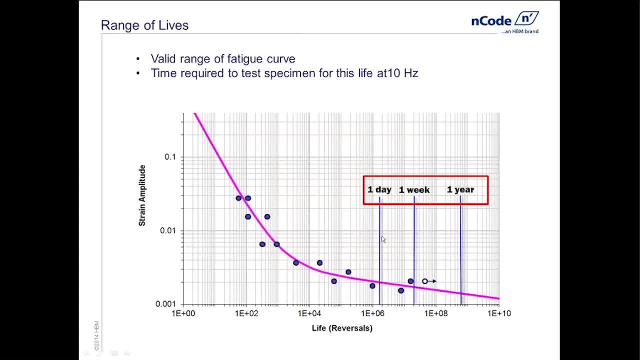 Cycles. It takes me a day to actually accumulate that test at 10 hertz, And 10 hertz is a reasonable speed for a strain life test. As we go out and try to get close to 10 million cycles, We're looking at a week on the machine. 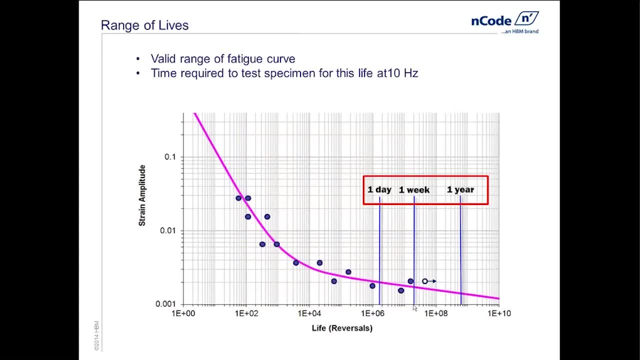 And again, if I were to push that out, to higher lives. We keep basically increasing the length of the test, So Having bounds on the high cycle regime Allows me to go off and make the most efficient test possible. Continuing with specifying the test. 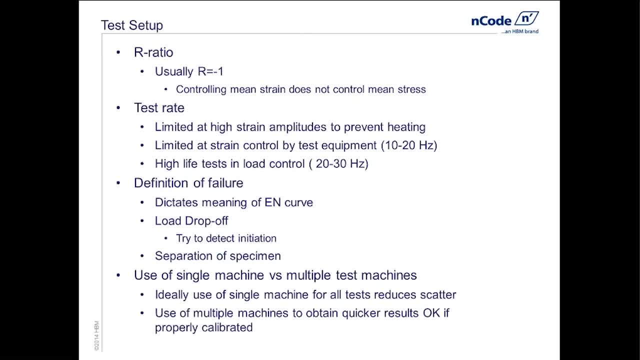 One thing that we need to specify is the mean strain that the test will be run at, And almost universally it will be at a mean strain of zero R minus one. And the reason for that: In stress life We may actually run tests at different mean stresses. 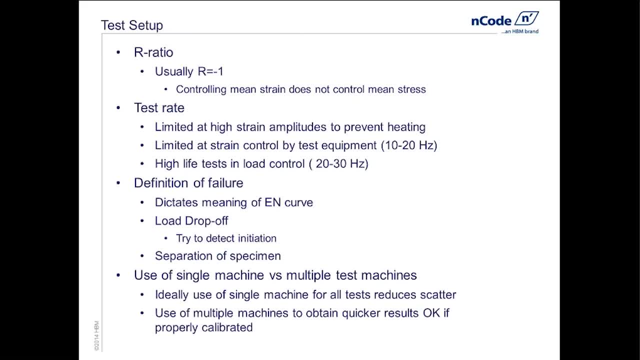 And that gives us curves that we could use. That may be far more accurate than an empirical mean stress correction Like Goodman or Kerber. However, In strain life, Mean strain and mean stress don't match up And at the higher load tests. 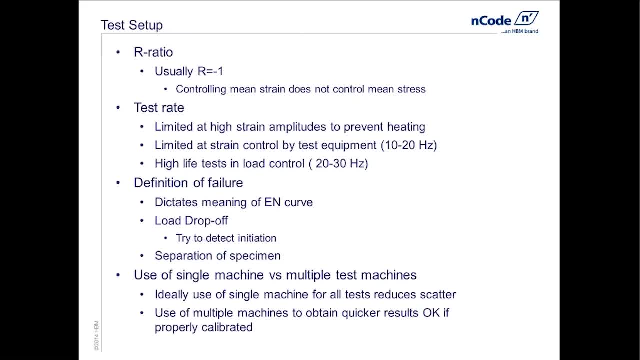 Even if I were to run at a different mean strain value, The mean stresses will start to move towards zero. So there's no control of the mean stress By mean strain. So almost invariably we're going to be running with a zero mean strain. 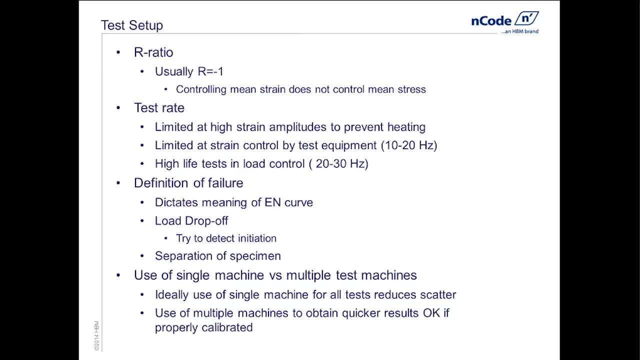 R minus one. With strain life. We're putting fairly large loads Into the specimens, Especially at the low life regimes, And so We want to pick speeds, Test speeds For our test rig. That will minimize any sort of part heating. 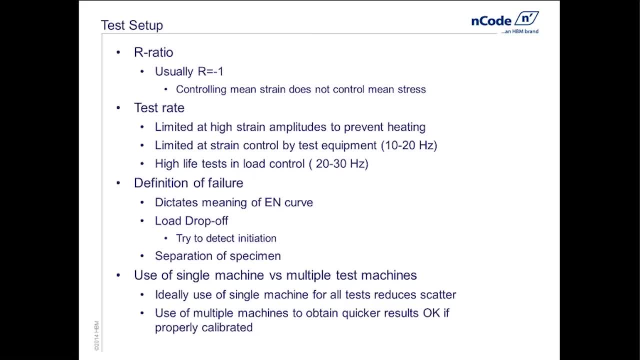 With metallic specimens We only have to worry about that for the fairly low life regime. But we want to basically control our speeds, So we keep a constant temperature on the specimen as we test it. In addition, These test rigs In reality. 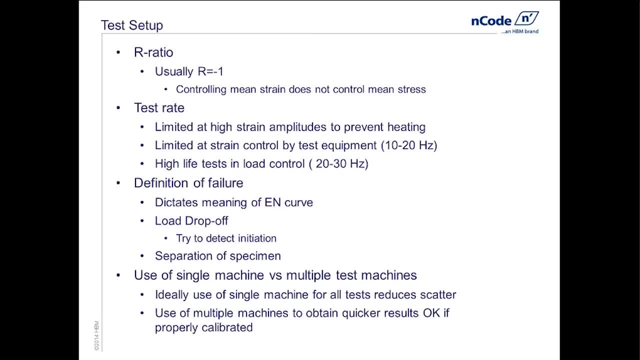 Are load control. That's how the test rig actually is activated, But we want to test our specimens Under displacement control Or strain control. In order to do that, We actually have to measure the strains on this test specimen And put it into a feedback loop. 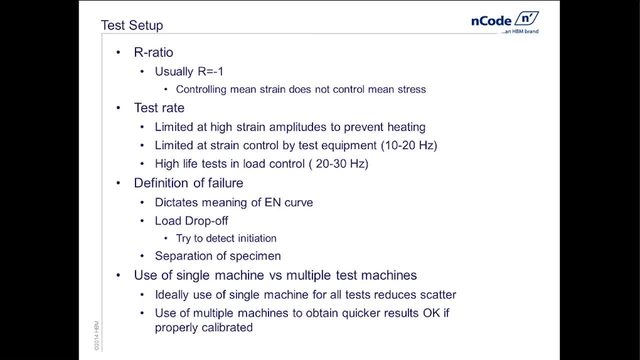 To control the load. So we always maintain the same strain That limits the speed that we can run at. So typically on a strain life test, You're running. If we don't have to worry about heating up the specimen. We're running somewhere between 10 and 20 hertz. 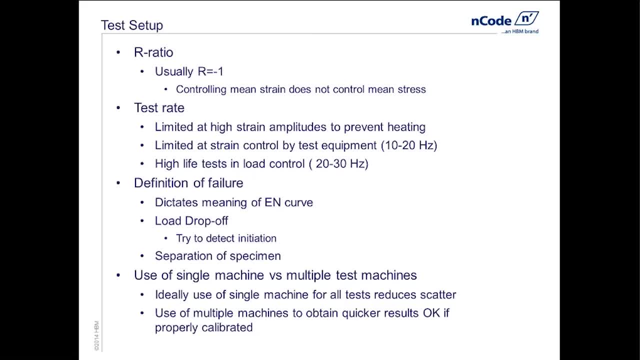 Now as we look at very high cycle For strain life Tests. There there's minimal plasticity And we can get away with Assuming that Load and displacement are the same thing. So you'll see a lot of times Test labs will go in. 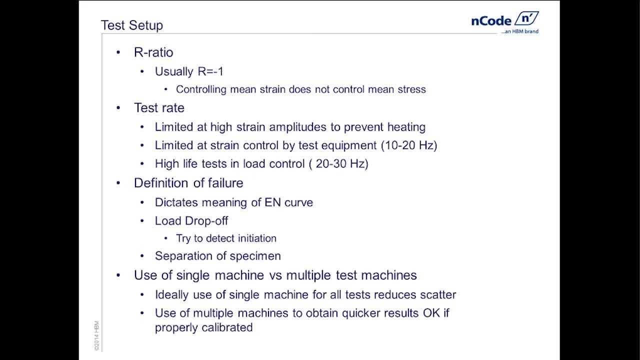 And at the higher life regime They'll go in, Switch over to load control And allow you to run at a higher speed. So we can at least up the speed of the test For those high cycle regimes And minimize any issues. 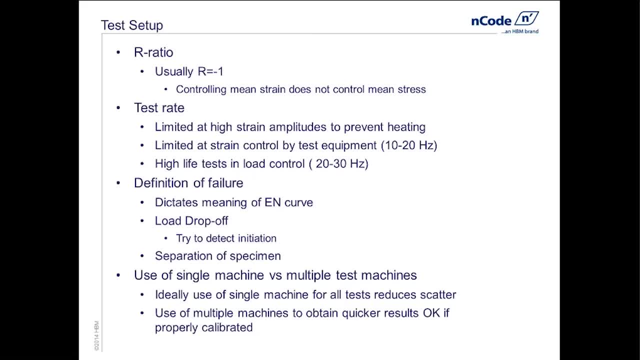 Because, again, There's minimal plasticity there, So we can get at higher speeds. One of the key things That you want to understand When you're looking at an SN curve Is what the definition of failure is That curve defines. 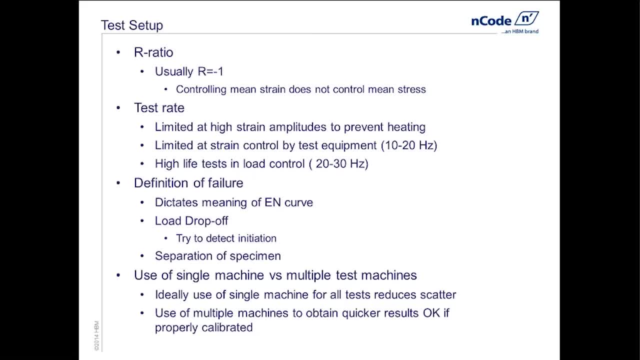 The part failed, But that can mean different things. It could be the fact That I have a load drop off. So I'm measuring the displacement Or load, And as the load drops off During the test, I have a particular percentage. 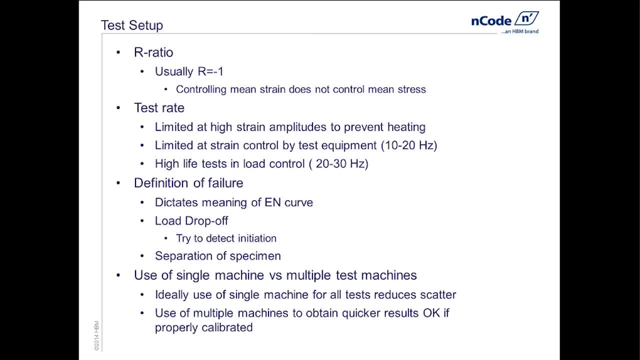 10%, 20%, That I say the part has failed. Again, That's kind of an indicator Of a macro crack in the part. Or it may be Pure separation of the specimen, But understanding that Gives me an understanding. 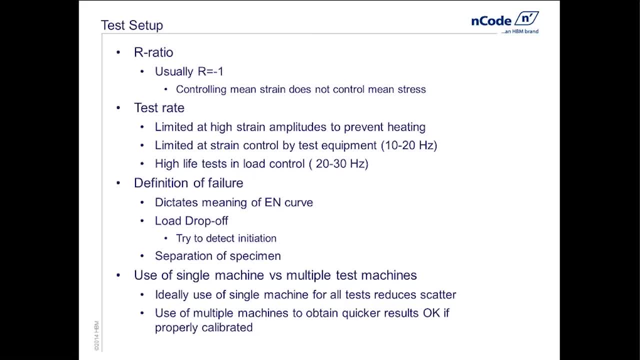 Of what the curve actually means. And the last Issue here: Ideally We're trying to, We're trying to minimize scatter Across the specimens So we can actually quantify The scatter in the material. Ideally, We'd like to: 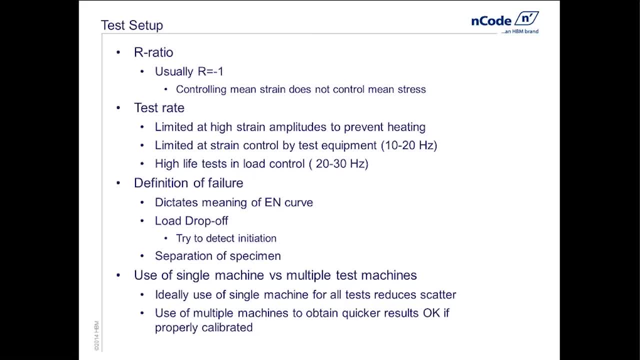 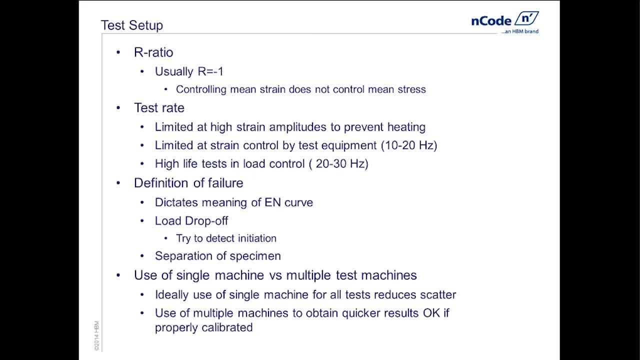 Ideal test. That would be the Ideal test. That would be the Ideal test. That would be. Yeah, I think it helps us Make those calculations. There's been a lot of good research. But There's been a lot of good research. 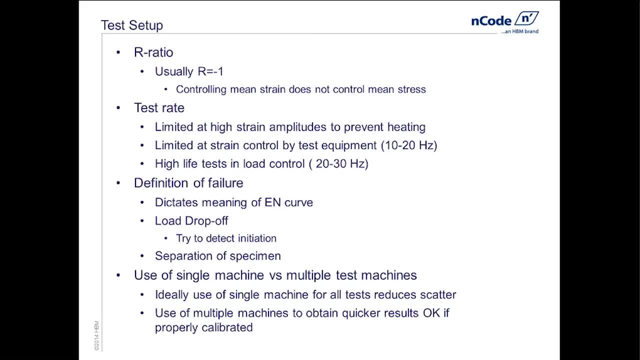 That really makes it Too ала. It's so hard That it's extremely Complicated. While I want to tell you, Go ahead, I just want To Please. We just want to close the episode with A few important things. 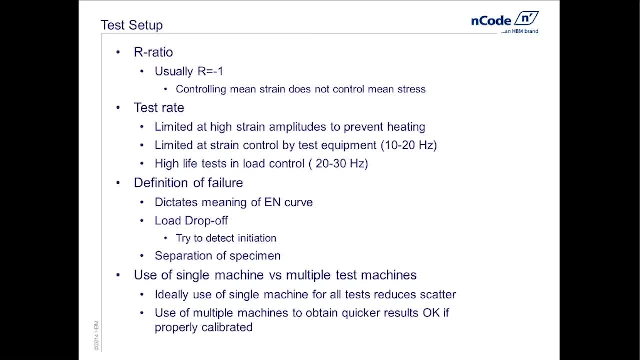 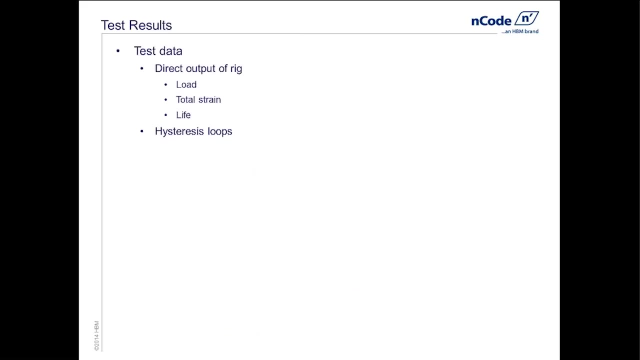 So Gin 돌아, Thank you for Being here And today. One of our스트 Access, Which are carefully prepared. Now We know Obvious due to the different machines. Once we've performed our tests, we now have data and the data can be in a couple forms. 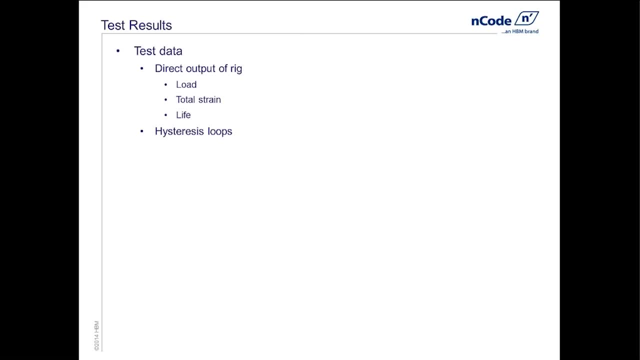 The direct output of the rig. the test rig we've seen is load, total strain and life Load. we're measuring. we're measuring the strain on the specimen and the part basically has a life. that is either the load drop-off or separation of specimens. 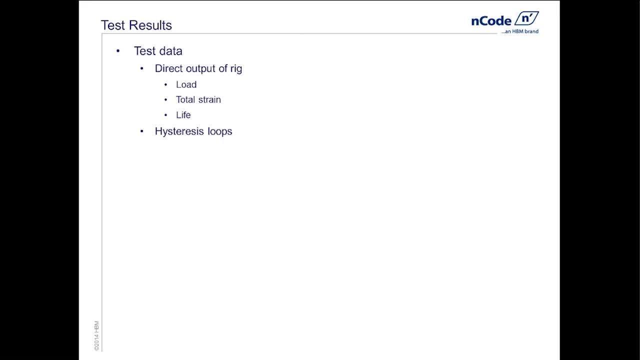 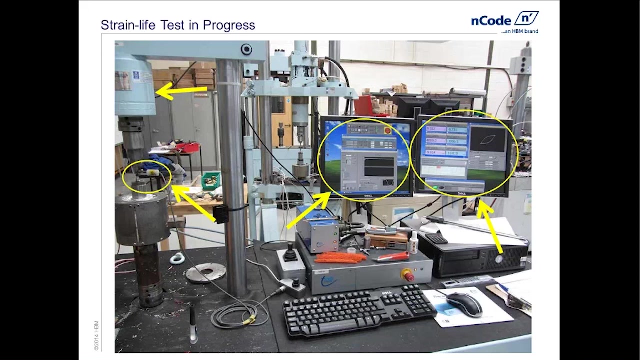 In addition, typically we are capturing enough data that we're measuring the hysteresis loops as well, so we're able to quantify the hysteresis loops. If I go off and look at just a standard test rig that we have here, what I have on the 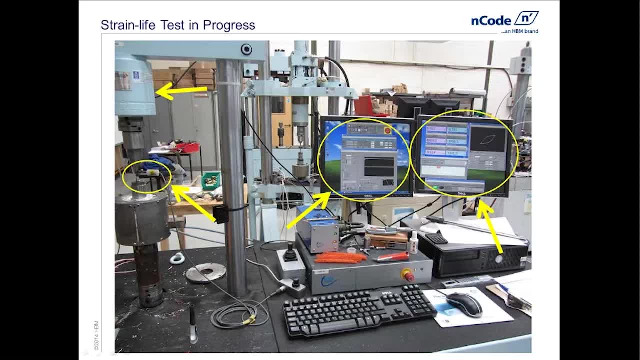 left-hand side is the actual rig. This upper section is the load cell That is measuring the load that's transferred to our specimen from the test rig. Our specimen is down here, gripped between these two grips, and attached to it is an. 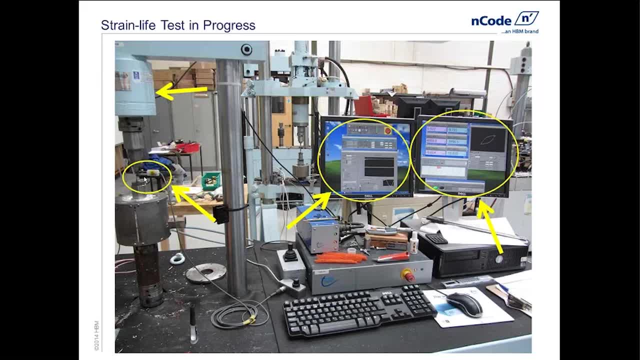 extensiometer. Basically it is an instrument that's clamped onto the specimen at the gauge length, measuring the strains that go on. We're actually just now looking at how much strain is there and how much load we have actually on that specimen as I load it. 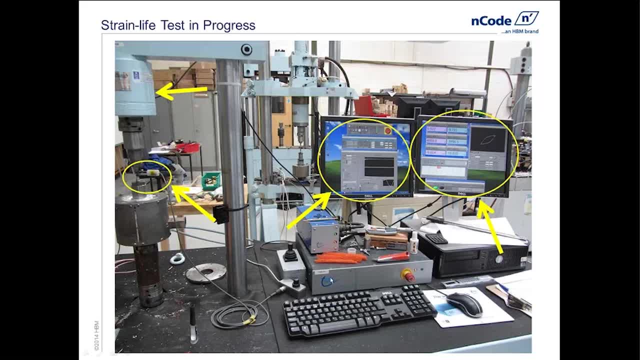 It actually feeds back to a controller that's controlling the rig. Again, we want to maintain constant strain on this specimen. We'll see in just a slide that the strain levels are not always tied to load levels. The other two circles here: The first circle is actually: 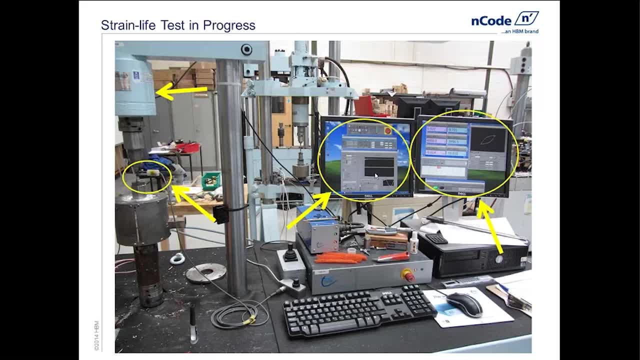 would have been a control unit, an analog control unit, today is being driven by a computer and so the display you see here, the CRT, is showing display of what would have been the analog control unit and this is actually driving the rig, basically maintaining a constant strain, going through, looking at the output of 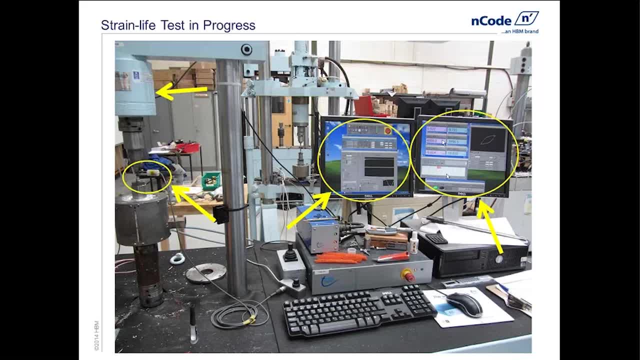 the strains from the specimen, and the second display is the data logger. this is actually collecting the data as we run the test. so we're actually tracking load total strain, but we're also able in most cases to go off and track the actual plasticity. the hysteresis loops coming from that and if you look at the 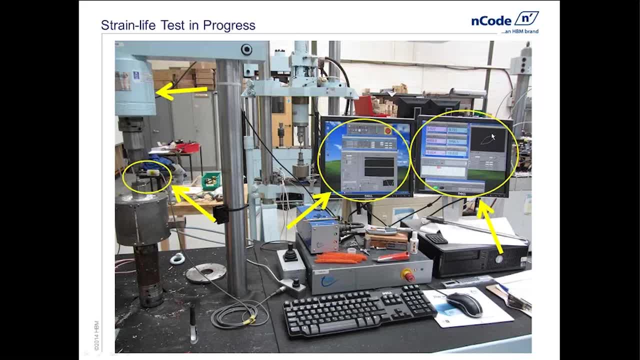 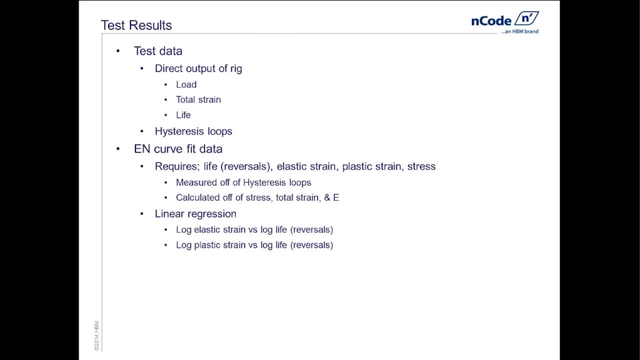 CRT, you can actually see the hysteresis loop that's currently being generated from the test. so with that data we then can go in and start to generate our strain life curve. and in order to generate the strain life curve, I need to have life. I also need to. 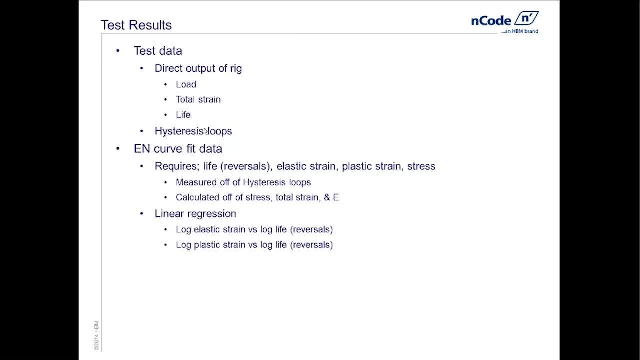 have elastic and plastic strain. those are the elements I actually need in my to do the regression for my strain life curve and I'm going to get that in one of a couple ways. I could actually synthesize that from load and total strain. if I know load, I know what the stress is in my part because of the 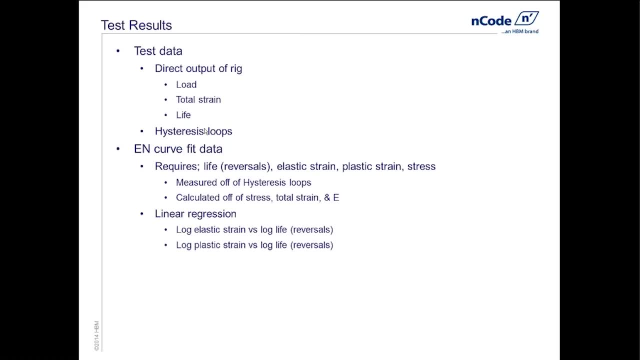 specimen geometry so I can dictate stress and if I know stress and Young's modules I can get the elastic strain that way. or we could actually go off and get the elastic and plastic strain directly off the hysteresis loops. if we're basically tracking those histories of loops, I'm able to go in plot a loop. 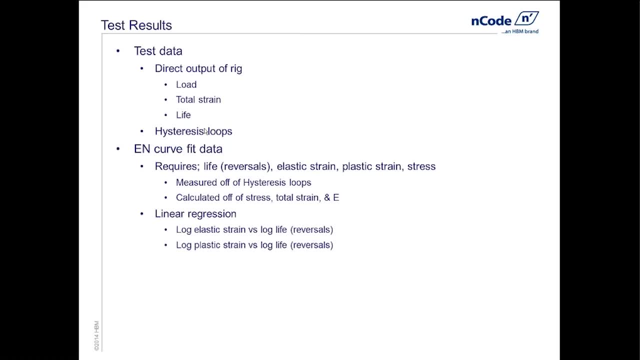 that's in a cyclically stable situation, Point in the test and measure off of it. We'll see that just a bit, So I have a couple ways to actually get the data. ideally we'd like to measure off the hysteresis loop and that would eliminate the any variation in the poison in the Young's modulus and 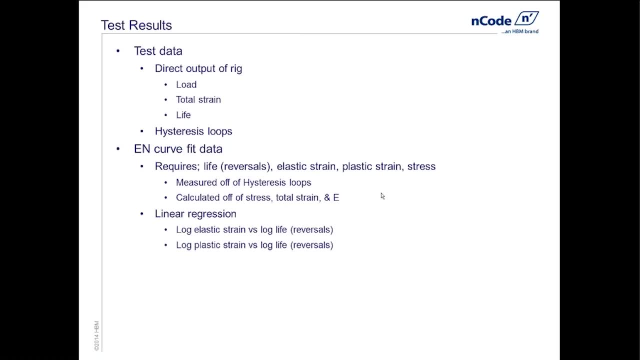 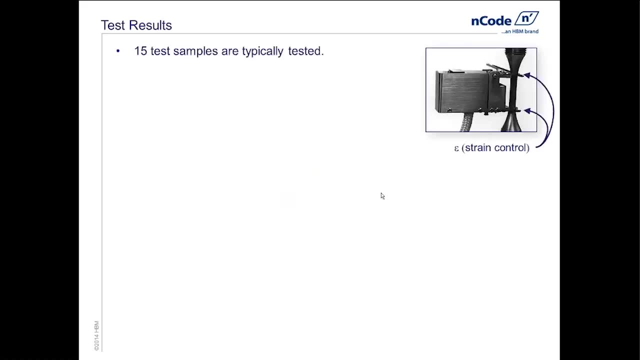 Then what we're going to do with that data is we're going to actually go off and do a linear regression through the elastic and plastic data, So Going off and looking at the coming out of the rig. again, We've had 15 samples. Each sample is run under strain control and again 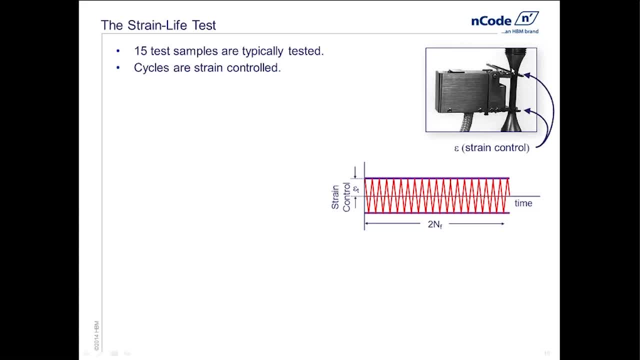 You're looking at a close-up here in this picture of that extensiometer measuring the gauge length, measuring the strains, and That feeds back into the test rig and the test rig is always maintaining that strain and If we look at a cycle We'll see that we can go in and track the load and the strain and 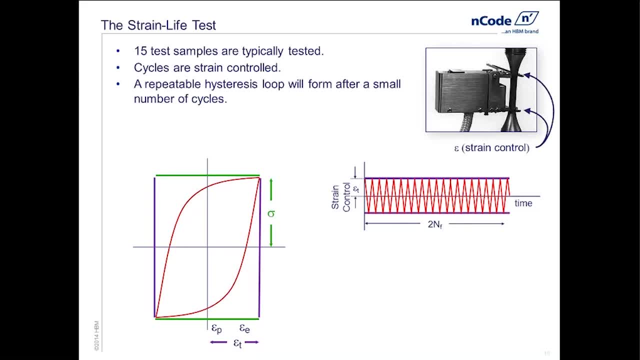 using that, we can actually predict these histories of loops. the load and specimen geometry give me the stress, and so I can start to basically track these histories of loops. The reason that we have a, that we have this fairly complex system, is that as we go through and cyclically, 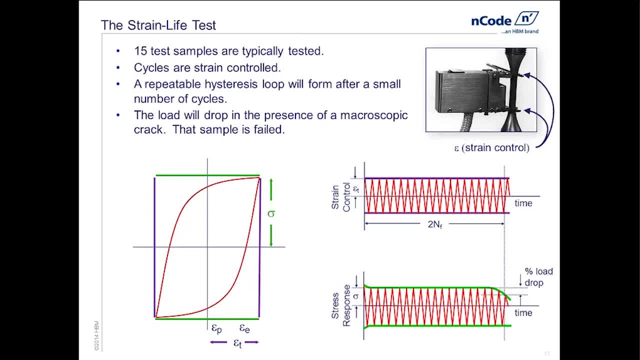 load these specimens, especially at the low life regime. we're basically developing plasticity. We're yielding the part and the actual material behavior changes. The first load on the part is following what's called a monotonic stress-strain curve. However, that behavior basically varies as we continue. 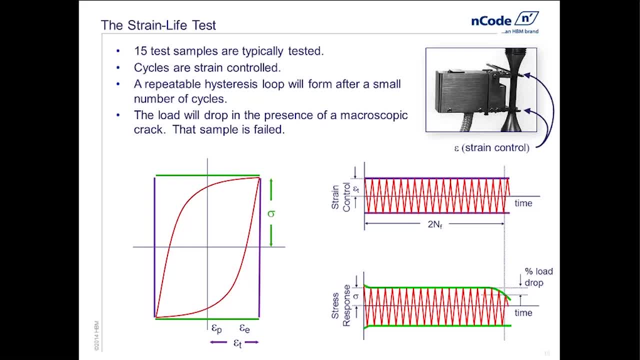 to cycle. After a few dozen cycles we will transition to what's called a cyclic stress-strain behavior, or stabilized Early on. the stress could be lower or higher than we would expect because we're on the monotonic curve, And then at the half-life, basically somewhere between the start and end of 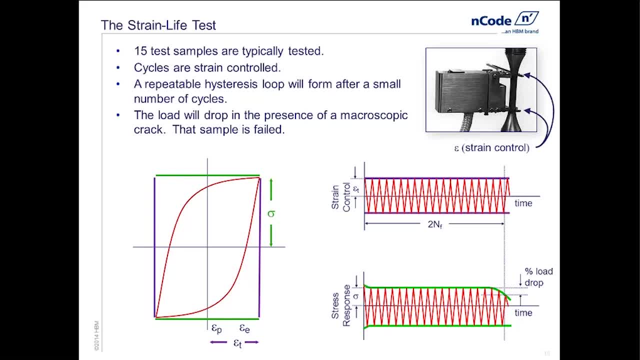 the middle, between the start and end of the test, we will have stabilized cycles And in that area we're going to pull out a hysteresis loop and that's the loop that we'll actually use to measure elastic and plastic strain. And again the 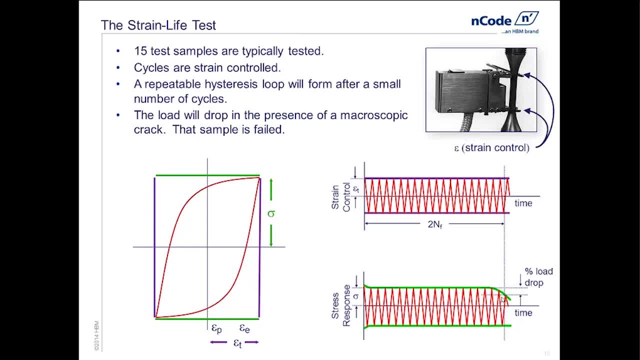 life is determined by the pre-determined either load drop-off or part separation. And so basically, from this we're going to get elastic and plastic strains and we'll get our life. So now we have elastic plastic and strains and life. One caveat: we talk about cycles and we also talk about reversals. The actual equation for strain life is reversals and there's two reversals per cycle. 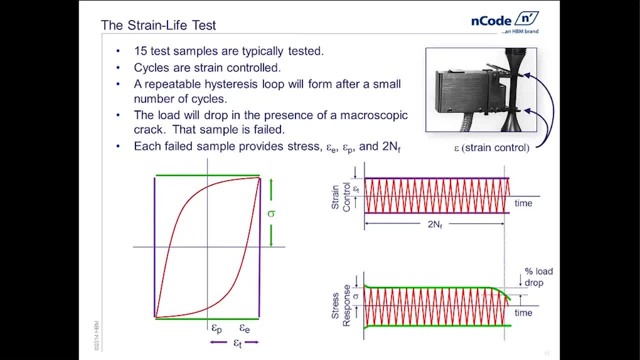 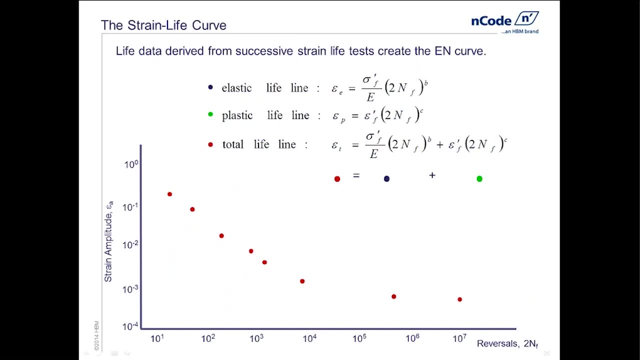 A reversal is just a change in direction of the loading, And so we're typically interested in cycles. but the equation itself is driven by 2NF, which means basically reversals. And here we see a series of test data. Those red dots are the total strain that were measured for different strain levels and each one is plotted. strain amplitude versus life in reversals. 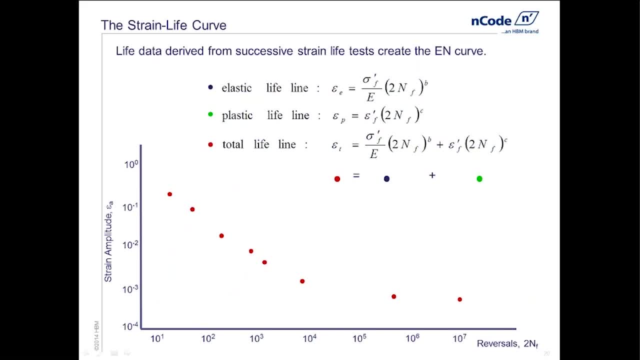 And if we look at the equations up here, the equation for the strain life curve is this bottom equation and it's comprised. the first component here is actually the elastic portion of the strain. So this is looking at elastic strains and it generates what would be a high cycle behavior. The second term here is looking at the plastic strains and it's basically driving the low cycle behavior. 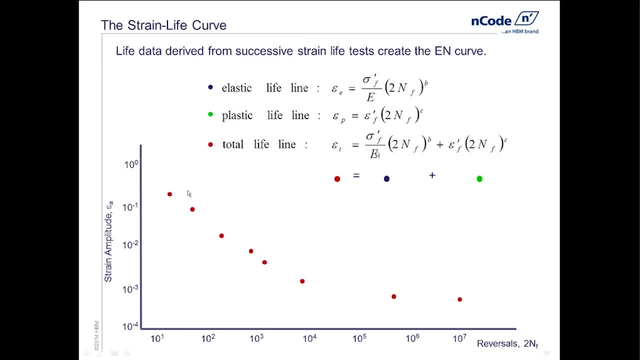 We don't actually fit this curve through these data points. What we do actually is take the total strains and we use either the load stress information or we measure directly off the hysteresis loop. But we basically dissect the total strain first into elastic strains. So now these are the elastic strains: elastic portion of the strain from the total. 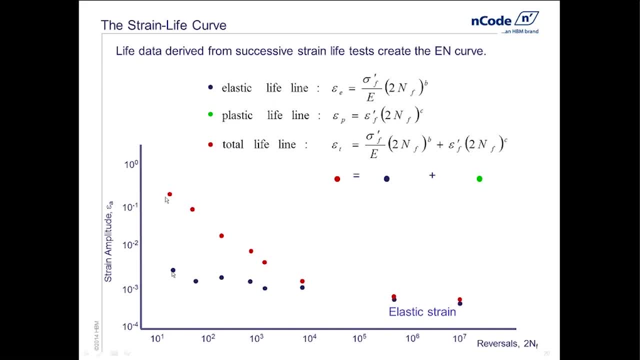 From the chose strain that was CFT3, we plug this intoользing tittiary. Slide 2 does the same哈哈哈. slide 1 does the same. slide 1 does the research slide 1.. All right, we plug these into a EMF chip. the functional must have an ins trailers. Here's a slide 1 view, nowhere in the slide around the visual diagram. we have to have everything classified in the visual graph. 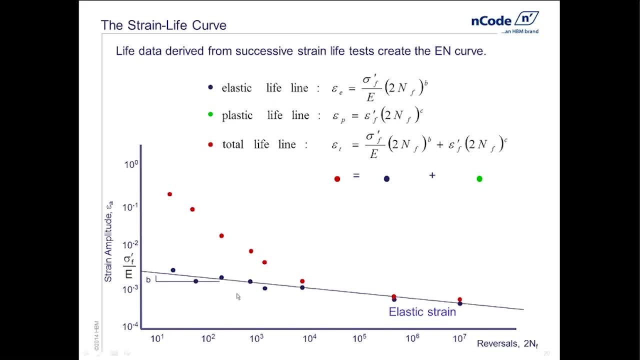 That worked well at the end of these sequences. but the most important thing about this example is this equation: as we're becoming very visited because we monsieur comes in through theデoscrypt elastic strains, we basically do a linear regression. again, this is on a log log. 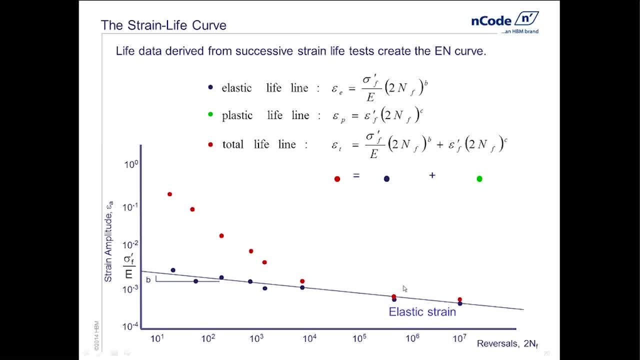 plot, and so we end up basically regressing. this we call the elastic line, or strength line, through the elastic data, and from this we get two parameters for the strain life equation. one is B, which is the slope of this elastic line, and the other is the intercept. the intercept is described in: 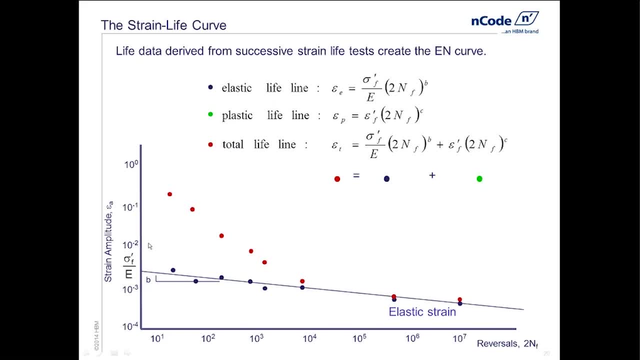 stress because it's elastic. we're just dividing by E, so it goes on the strain axis, which is the vertical at vertical axis. so the Sigma F, prime and B are the parameters for the high cycle behavior. in addition, we take and we also extract the plastic strains from the total and we regress a second line through that. so 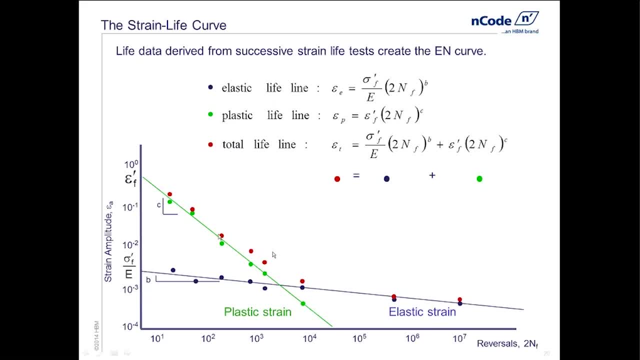 that green line, there is the plastic line or the ductility curve, and again it provides two more pieces of data: C here is the slope of that and epsilon F prime is the intercept and those four pieces of data, B and C as the slopes, and Sigma F prime. 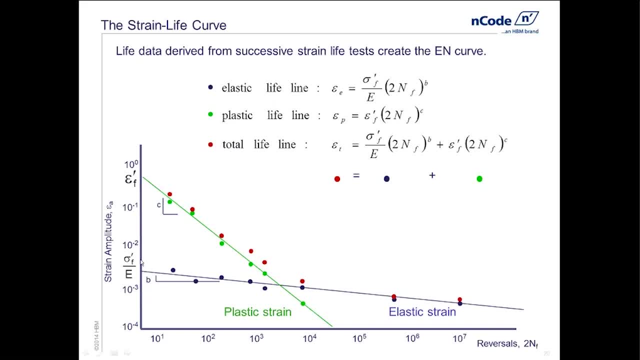 and epsilon F prime basically are the components that parameters. I need to describe the strain life curve. so the strain life curve actually is the addition of those two straight curves in log log space. so we're going to actually do our with this red curve. the total, basically this is the actual strain life curve, but 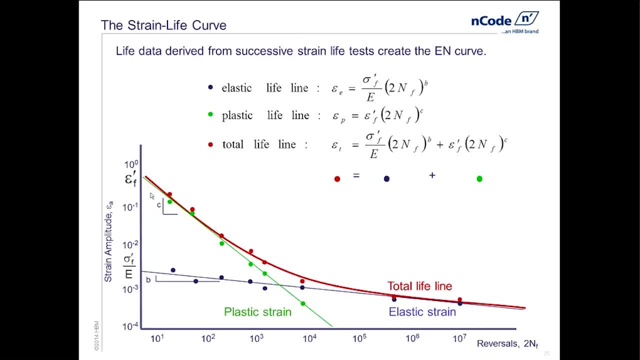 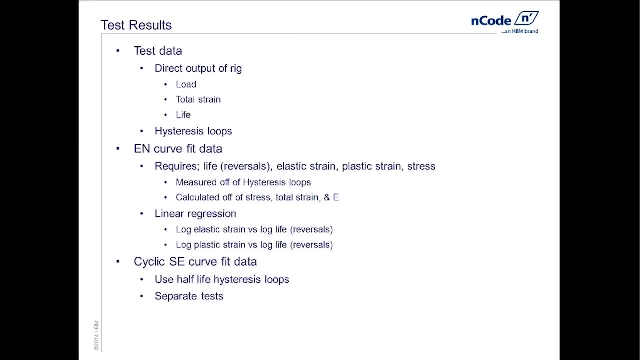 it is actually computed from separate regressions to elastic and plastic strains. because we're interested in plasticity, we need to have stress strain behavior as well. many times, especially for moderate, moderately low to high cycle behavior, plasticity is done inside of the fatigue program, which means we 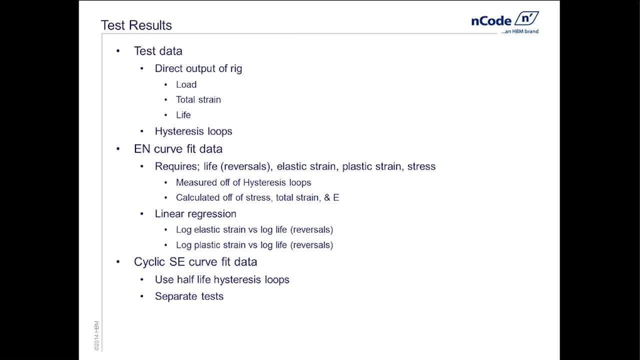 have to have a stress-strain curve there to do our fatigue calculations if we're at very low lives. we need to do the plasticity in the final program, but we still need to have stress-strain behavior there as well. so we need to get the stress-strain behavior there as well. so we need to get the stress-strain. 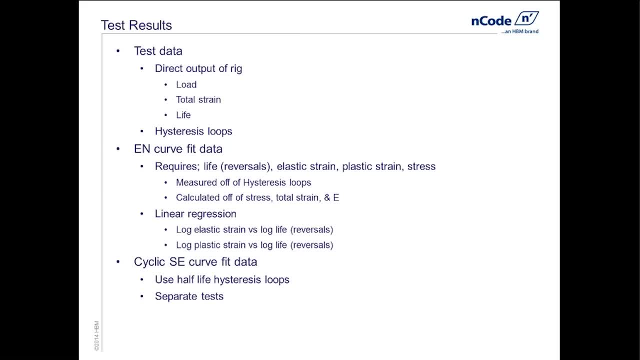 curve defined and there's two ways to do it. we could calculate it directly off of the hysteresis loops that are being collected as we do the test, and again we take those that histories loop from half-life, you know basically somewhere in the middle of the test. so we have stabilized behavior, or it can actually. 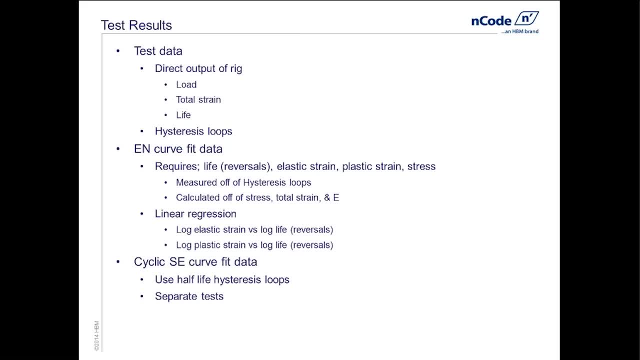 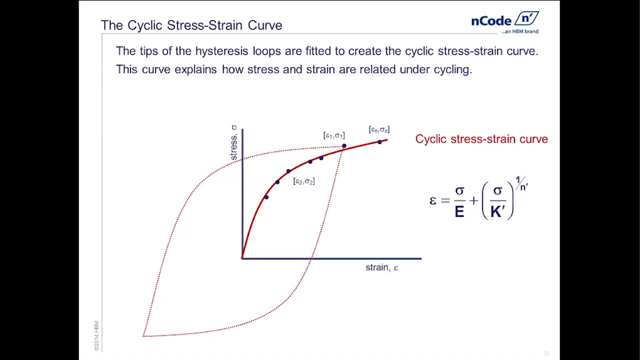 be done in separate tests. so we can either utilize the fatigue tests data to do the regression or we can- actually we can- go off and do separate tests. in our lab we tend to use the fatigue tests. however, I have had customers that feel that they can go off and have more flexibility in running separate tests. 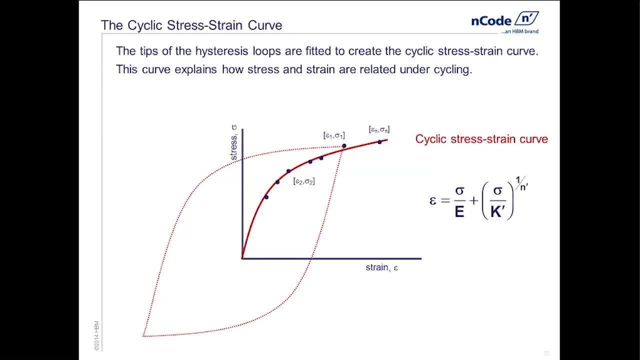 with to get the stress-strain behavior if we're. if we're going in and using the fatigue test to generate this curve, what we're actually going to do is we're going to have a whole family of history sys curves, each one of these at a 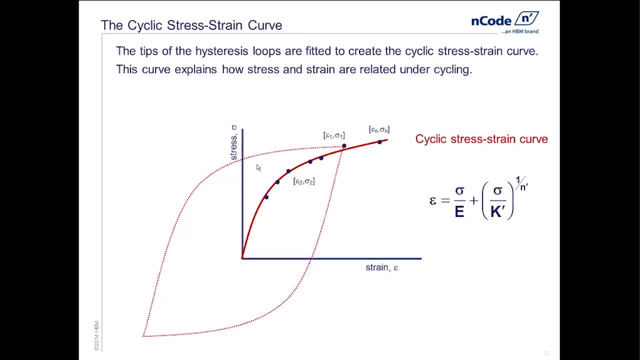 different strain level and so at the little you know at the beginning of the know, at the lower strains of smaller hysteresis curves, and as we have higher strains become larger and what we do is we pick the, the upper corner of the hysteresis curve and that point is used as a stress strain value on my stress. 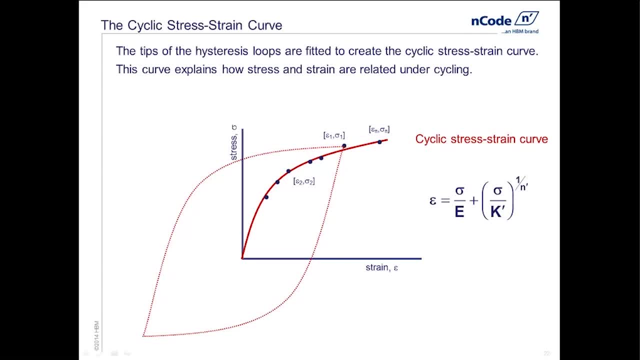 strain curve. so what you're looking at here, these blue dots, are basically this upper vertex of the hysteresis loop for different load levels, and what we're going to do is regress a curve. through that the stress-strain behavior that we use for fatigue is written as a Ramberg Osgood equation, which is nothing more. 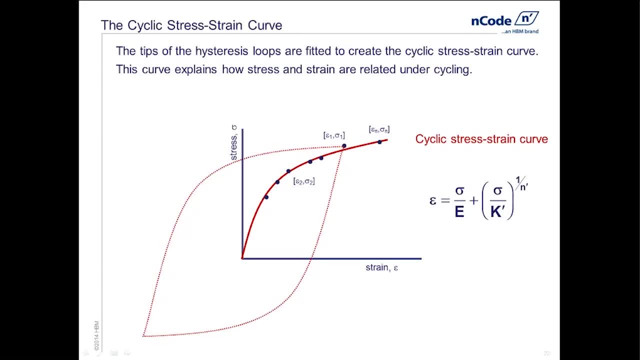 than saying that the strain is elastic part and plastic and this plastic piece right here is nothing more than a straight line curve in log, log space of plastic strain and stress. so we basically are going to take these points, go through these points and we're going to take these points and we're going to. 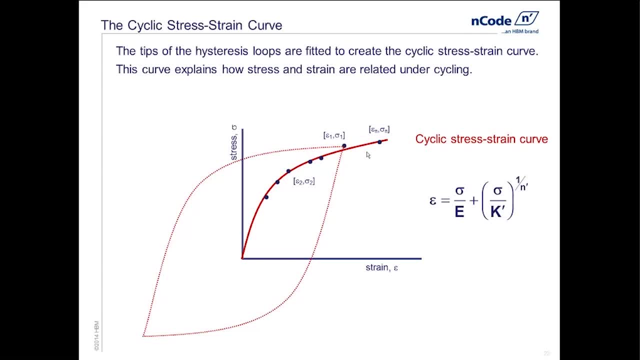 go in plot the plastic portion of the strains on log log curve and just get a light straight line through this. and n is the slope of the curve and K prime. n prime is the slope of the curve and K prime is the intercept at a strain of one. 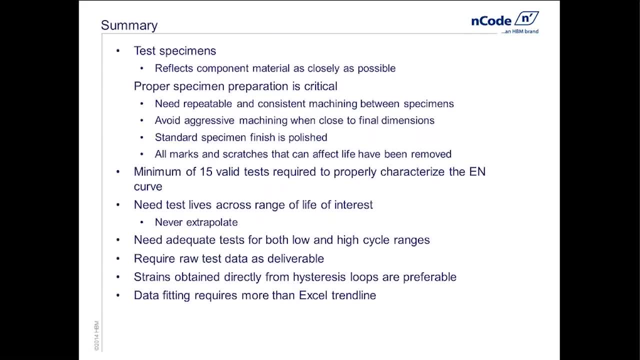 so with the stress strain behavior, the cycle of the, the cyclically stable stress strain behavior, stress strain curve and the strain life curve, we now have an updated harmonic analysis for our sample, once we go off into a crack: initiation fatigue analysis. so, in summary, walk through the steps. we've talked about the things that we had. 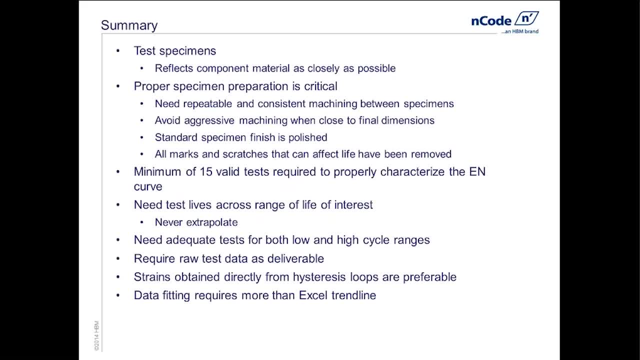 to kind of at least answer questions to the test lab that were, or to our internal test lab for a company, things that we need to worry about again, the test specimens, and again we want the specimens to be mature. So we're going to go off to these type notes and then go through the situation that came as well. 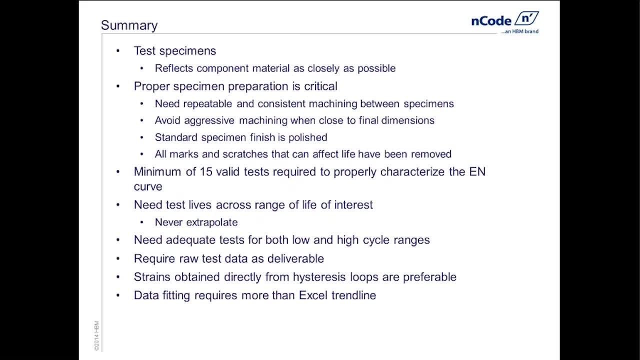 made of material that, as closely as possible, represents the material of our part, composition, microstructure, heat treat. The preparation of the specimens is critical. We want to guarantee that when we end up with a specimen, that it's dimensionally correct, so there's no variation across, minimal variation across specimens, as well as it's a geometry. 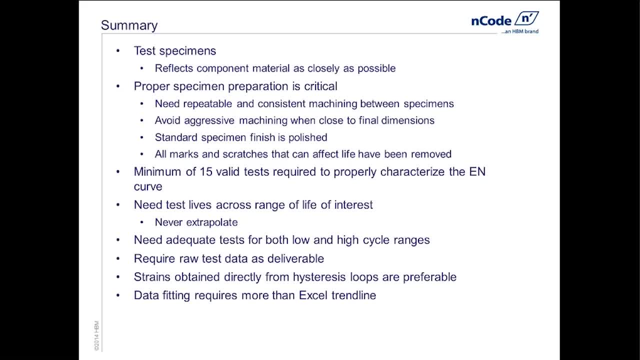 that as I apply a tension load, I'm not inducing things like bending because of misalignment of the specimen. I want to control the final surface, finish on the specimen and when we say polish it's not like a mirror. I see myself in the specimen but we want to eliminate any machine marks, scratches. 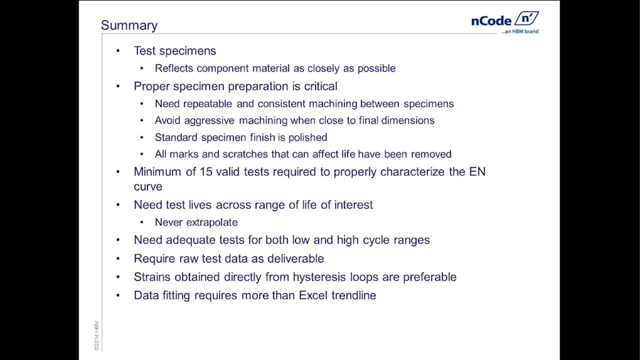 that would be initiation points for that. In terms of number of tests, we want a minimum of 15 tests to do a baseline curve and actually 20 to 25 would be better. Again, the more specimens, the higher the confidence level, the less conservative the 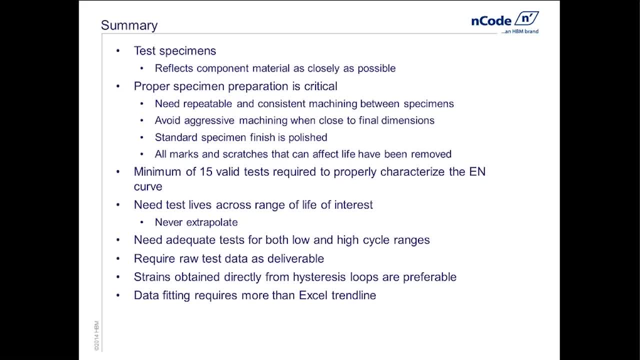